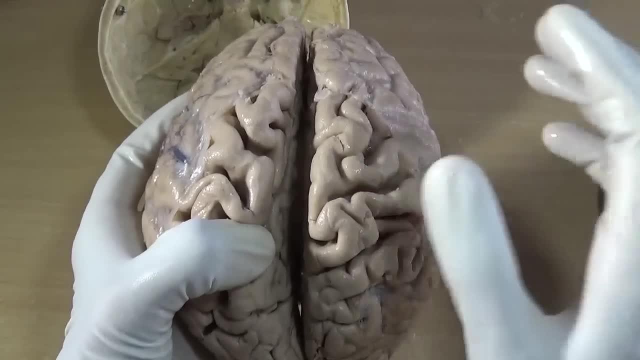 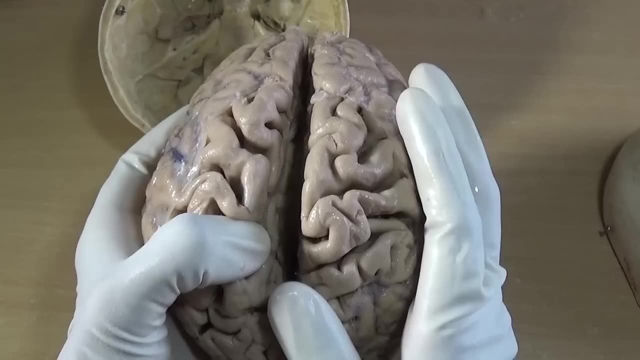 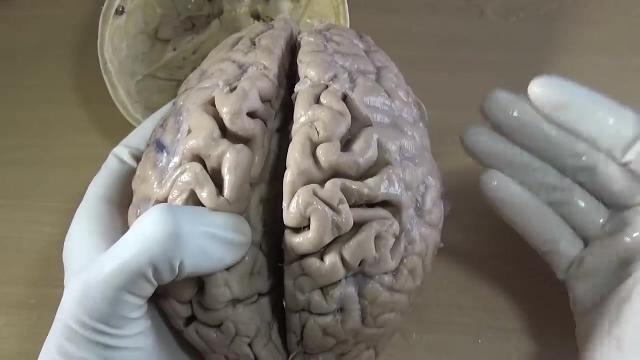 that is termed as basal nuclei. so by and large, the cerebrum is made up of three structures: outermost cerebral cortex. second layer is the white matter. that is nothing but the axons or the fibers running across the cerebral hemisphere or from higher center to lower. 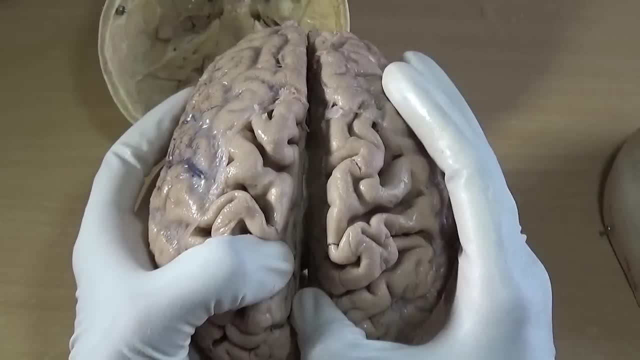 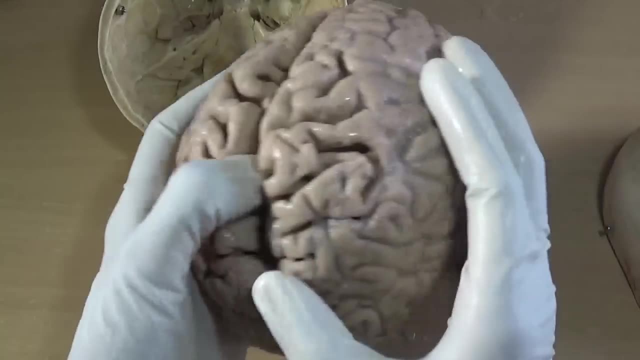 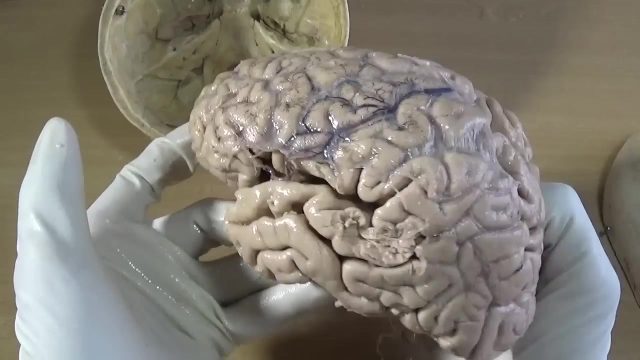 center or across the midline, and the innermost gray matter is in the form of basal nuclei. so this is what you see from the surface is cerebral cortex which is having convolutions, which is having elevations and depressions, and these are termed as sulcai and gynecomastia. 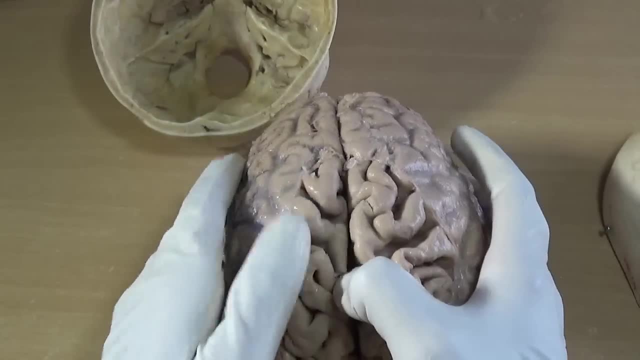 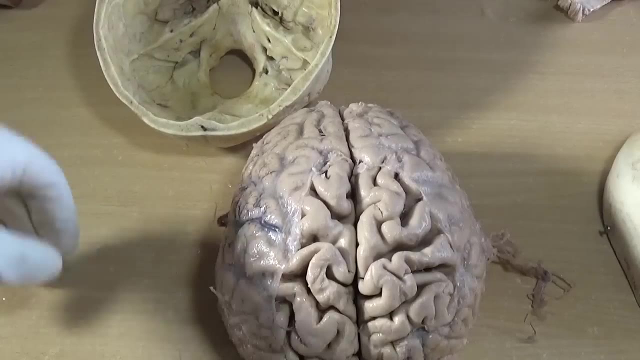 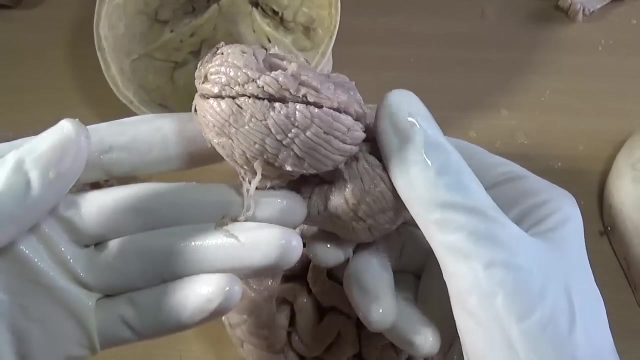 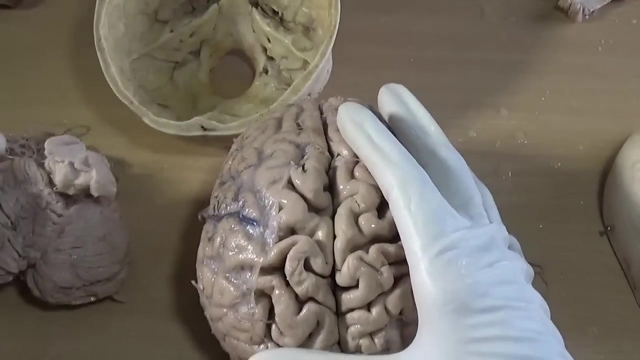 gyri, so what you call fissures and folia in case of cerebellum. let me show you. see, this is the cerebellum. so here also there are elevations and depressions. these are termed as fissures and folia. so depressions are fissures and elevations are folia. similarly over here. 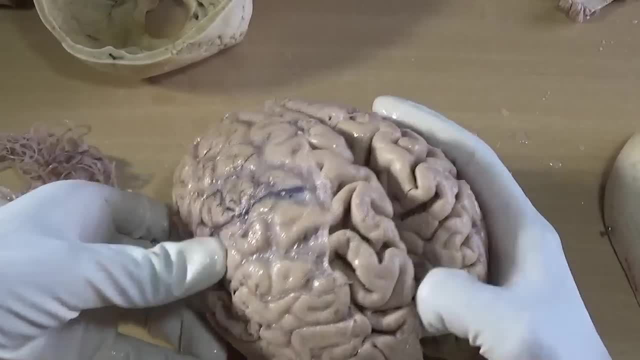 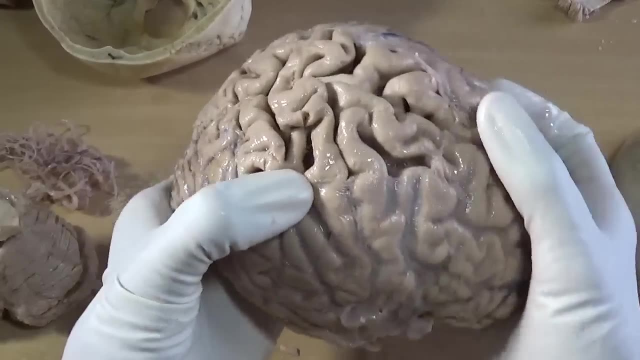 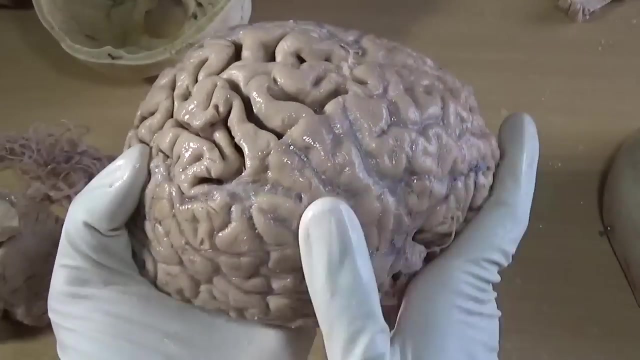 also the depressions are termed as sulcai and elevations are termed as gyri. so when you see such type of the cerebral cortex or cerebrum, then it is termed as gyrancephalic type of the brain. that means it is having surface convolutions, irregularities and particularly 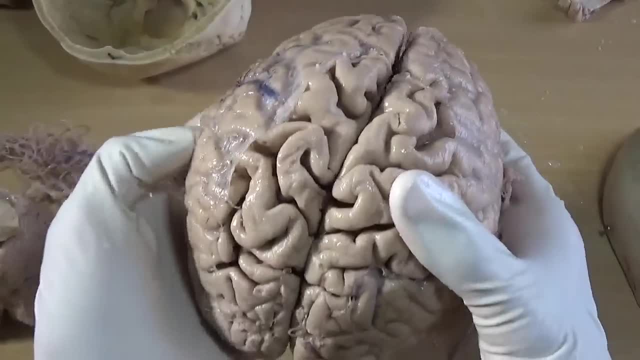 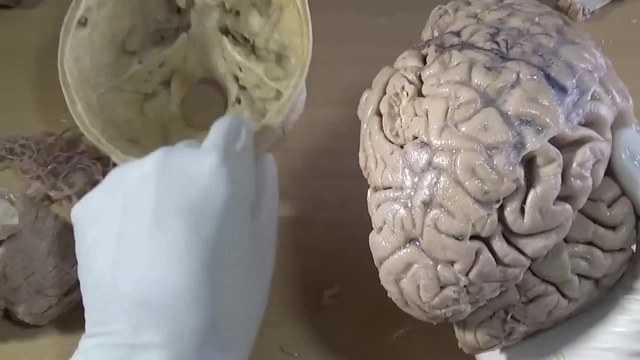 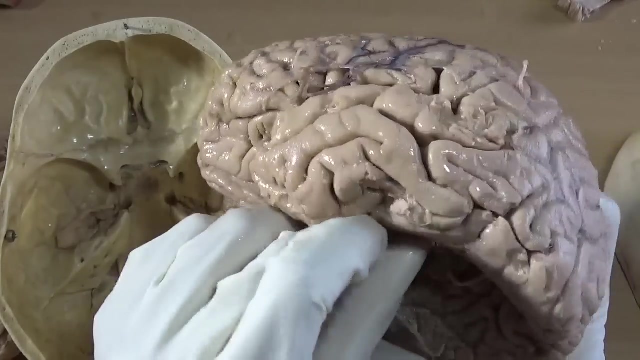 in case of human being, there are maximum such gyri and sulcai. it is just because, to accommodate the large surface area within this brain box, it is said that two third of the surface area of cerebral cortex is hidden within the sulcai. see this and what you see over the surface. 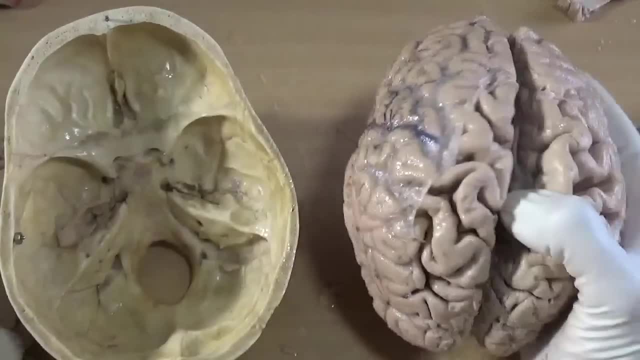 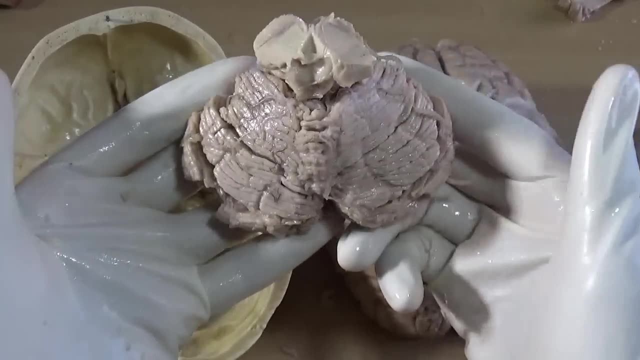 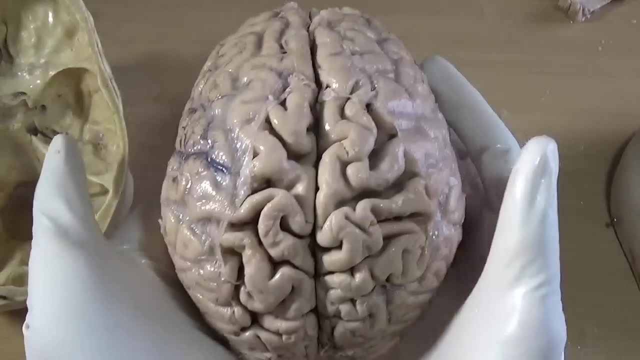 is just one third of the surface area. on the contrary, for the cerebellum 85% of the surface area is hidden within the fissures and what you see on the surface is just 15% of the surface area. so human brain is having gyrancephalic type of the brain, or human is a gyrancephalic. 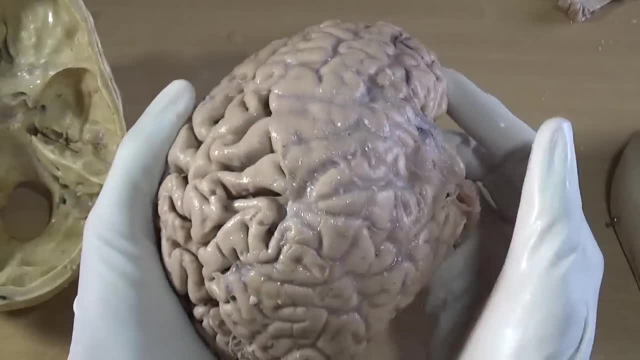 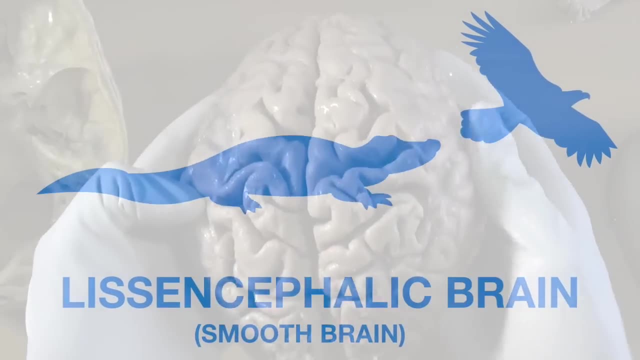 but in case of lower animals, lower mammals or even animals, which is the subcutaneous tissue of the brain, you will see that the subcutaneous tissue is located within the surface area of, say, for example, birds or reptiles. they are having minimum surface area and they don't need such 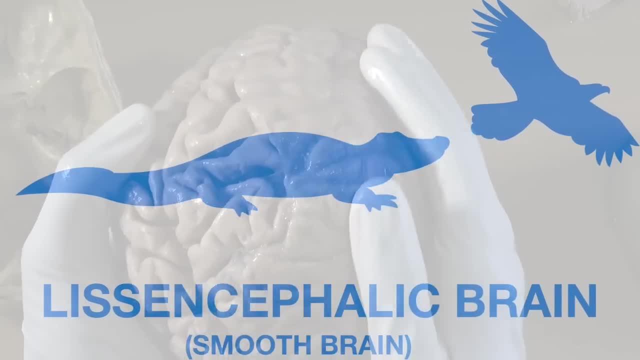 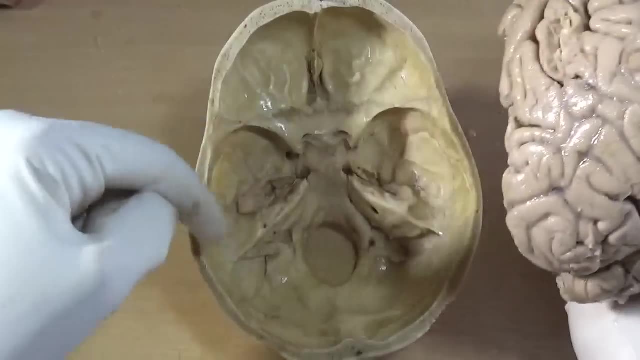 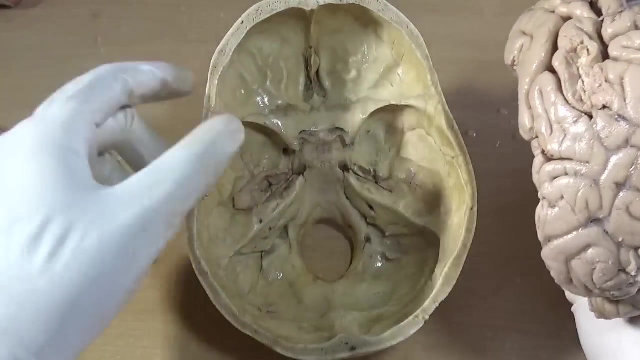 gyri and sulci, so they have got a smooth cerebral cortex and they are termed as lisencephalic. now you know, it is fixed within this cranial cavity and it is divided into anterior, middle and posterior cranial fossa. so accordingly, according to this three cranial fossa, there are 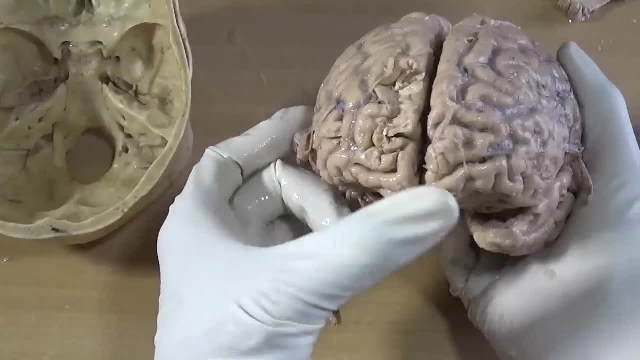 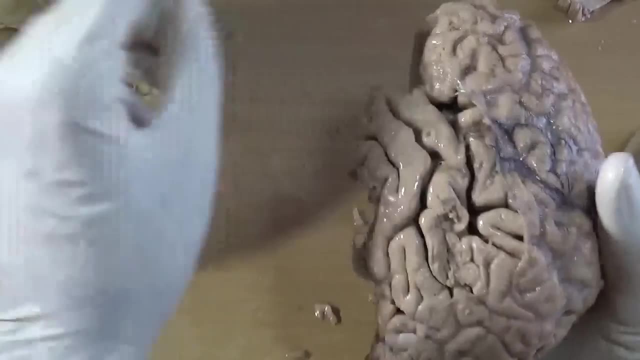 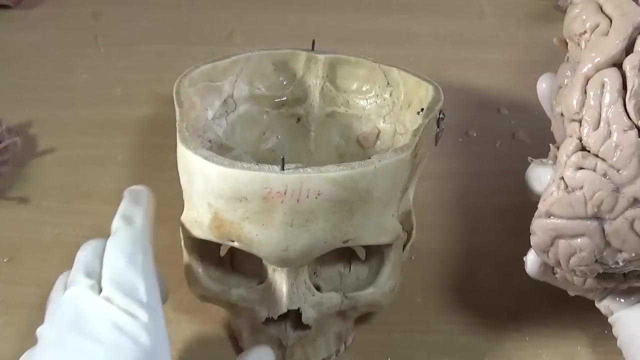 three poles: frontal pole- see this, this is the frontal pole. then there is a temporal pole and then there is an occipital pole. so accordingly, the frontal pole lodges in the anterior cranial fossa, particularly if you see it from in front. this is termed as super ciliary arch. so exactly, 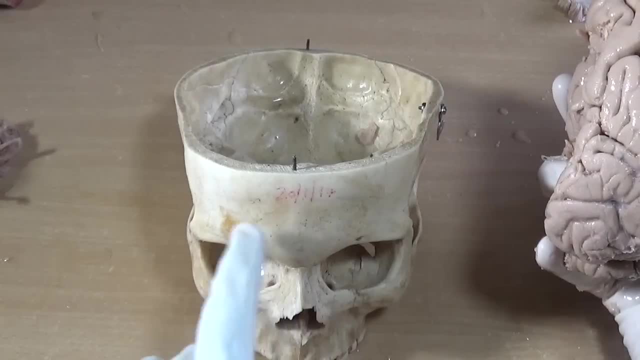 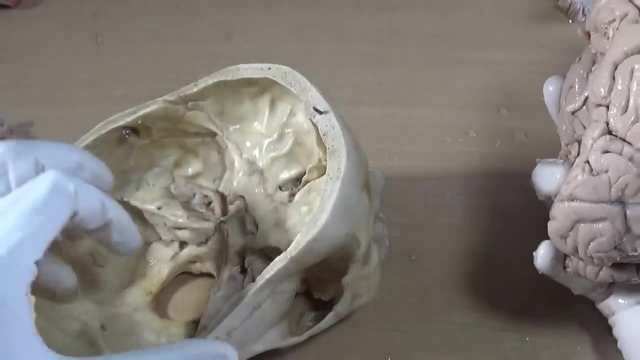 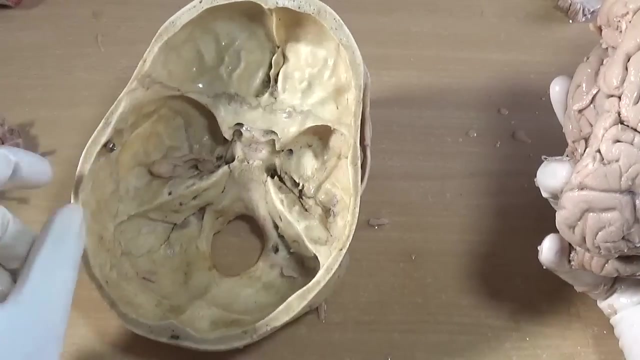 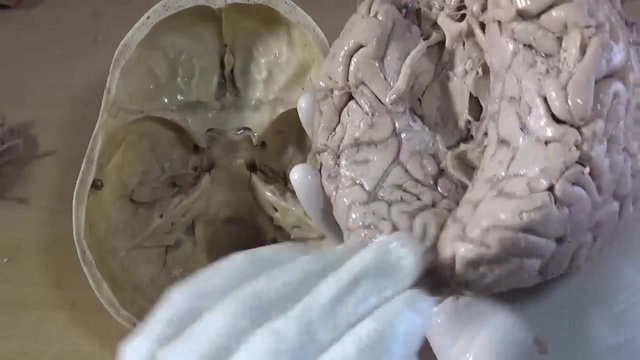 just medial over here, supramedial to this super ciliary arch over here, just behind to this point, we will get this frontal pole, the temporal pole lodging temporal lobe is found within this middle cranial fossa and occipital pole is resting over the tentorium cerebelli over here, this portion and this is the occipital pole. so 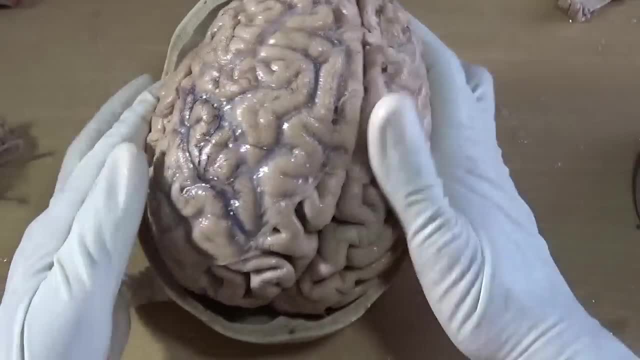 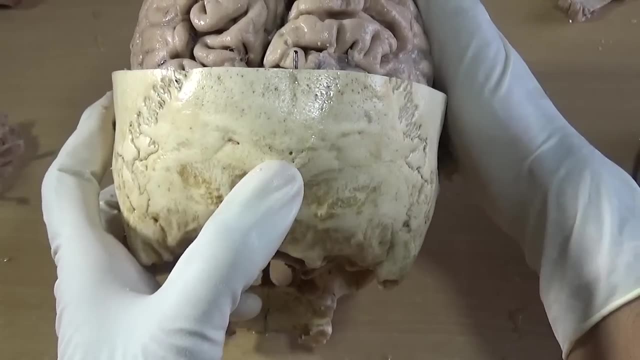 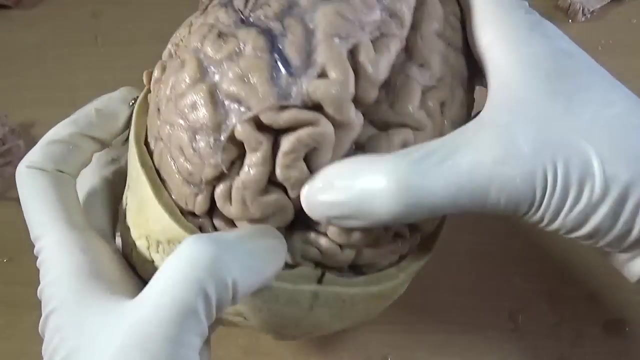 when you imagine occipital pole found embedded within the cranial cavity. so this is the external occipital protuberance, so just supramaterial to this external occipital protuberance, deep inside there will be occipital pole. so this is how three poles of 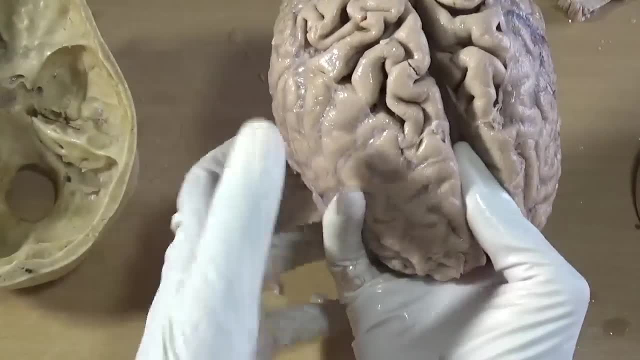 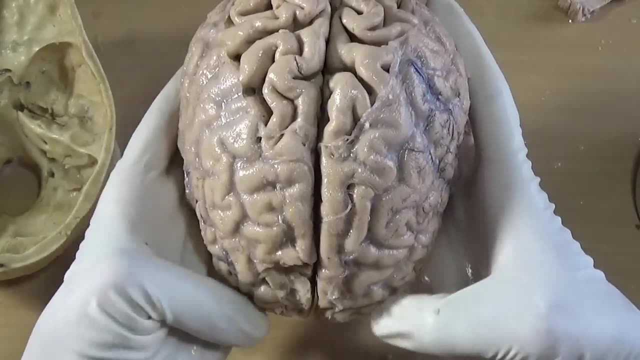 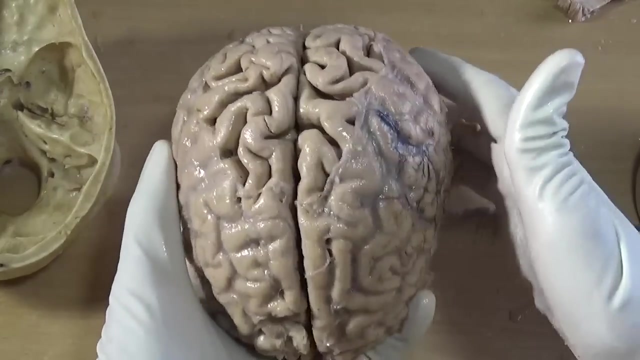 the cerebral hemispheres are accommodated within the cranial cavity. now, when you see it from above, the anterior end is tapered somewhat and along the posterior half you will get the maximum transverse diameter that is found underneath the parietal tuberosities. so by and large, you can get surface diameter that is oval in shape, it is not circular. this is anterior end and this is posterior end, and when you see the frontal poles, they are more or less rounded. as compared to the occipital poles, they are more or less pointed. so this is how, from above, from external aspect, you can differentiate which one is the anterior end, which one is the posterior end, and obviously the temporal pole is directed forward, so that too will help you to determine the lateral movement direction. 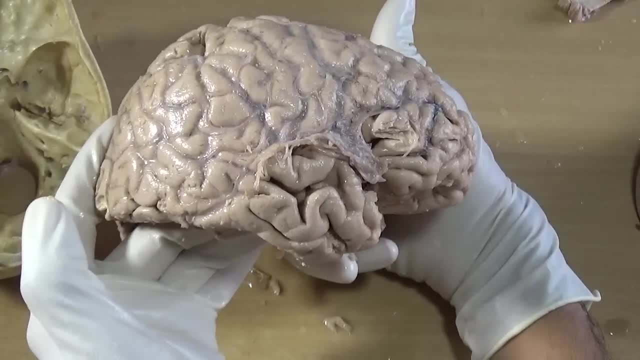 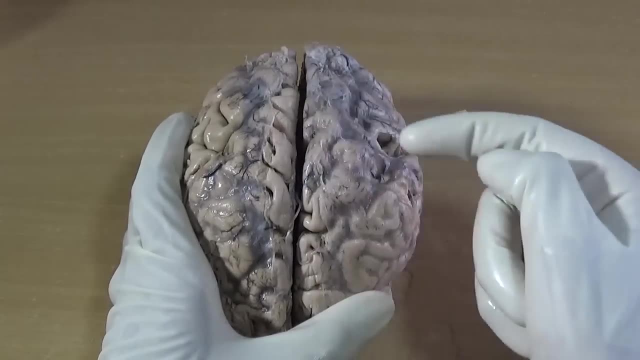 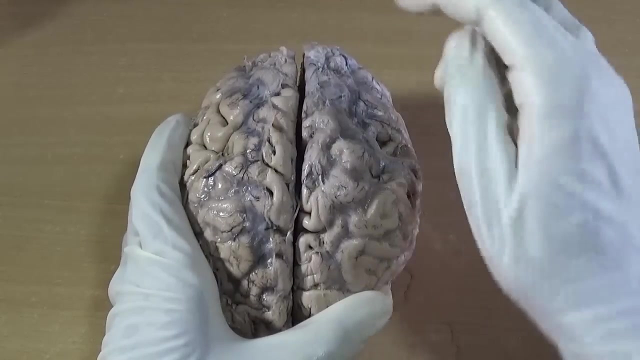 anterior and posterior pole or anterior and posterior aspect of the cerebrum. So this is median longitudinal fissure and deep inside, as we have discussed, there is a largest bundle of commissural fiber, that is, corpus callosum, holding these two cerebral hemispheres together and within, 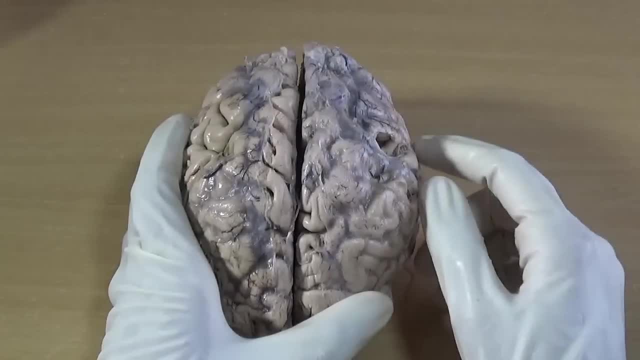 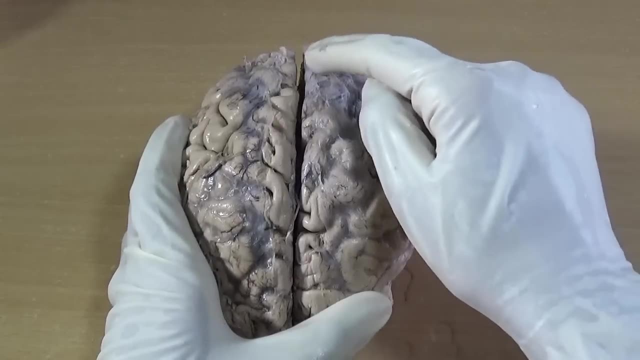 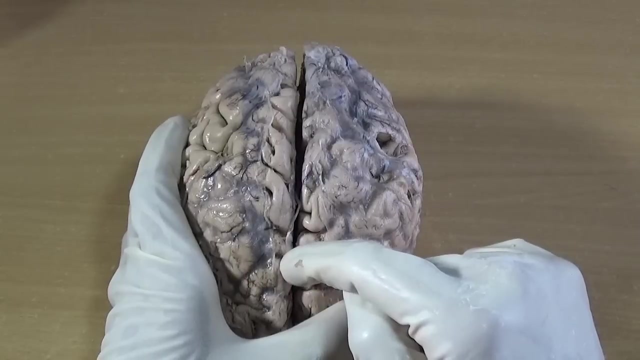 this fissure it lodges a fold of dura mater, that is farc cerebri. Within the farc cerebri there will be superior and inferior sagittal sinuses. Along with the fold of dura mater, this fissure lodges a fold of arachnoid, and pia mater, as well as anterior cerebral vessels are found deep inside. 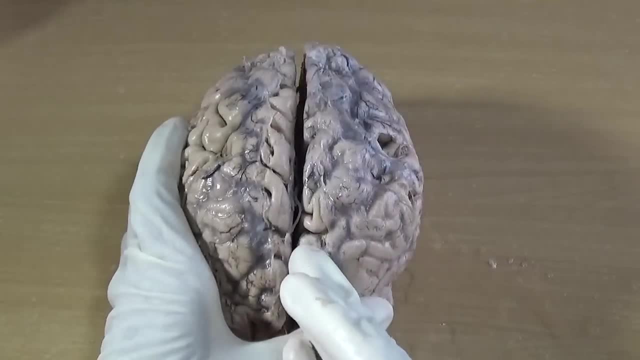 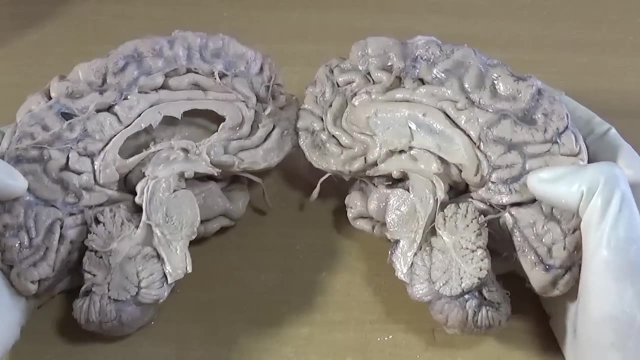 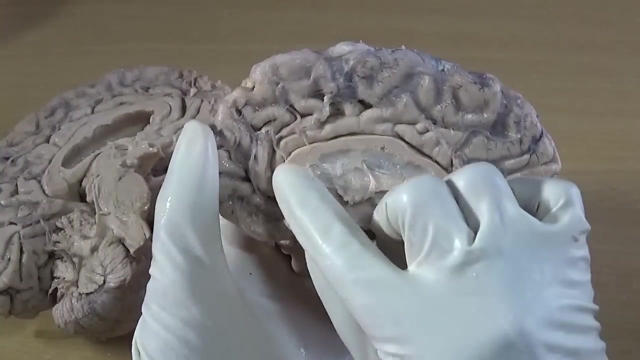 Now, when we cut open through this corpus callosum and when we expose it, this is how it looks like. So these two are now cerebral hemispheres and this is how it looks like And this is what we were discussing. this is the largest bundle of commissural fibers, that is. 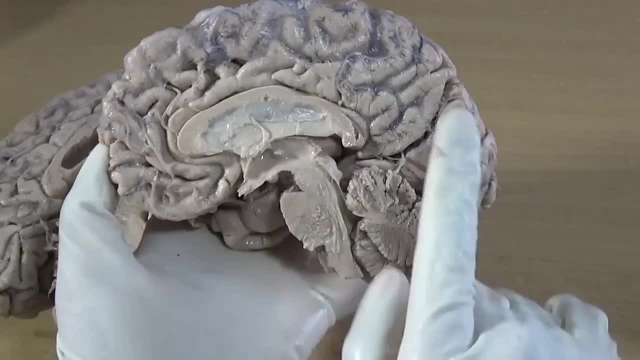 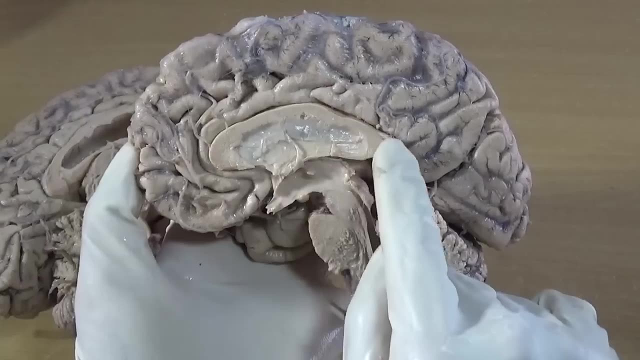 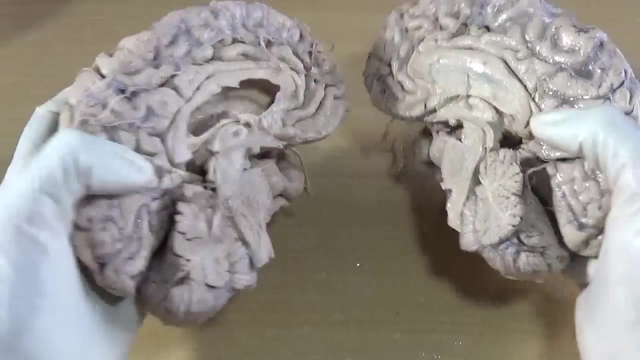 termed as corpus callosum. So from in front, from behind, the cerebral hemispheres are separated from each other, but from the center they are connected by this corpus callosum. So this is right and this one is left cerebral hemisphere and this is how they are connected. So we have cut them open. 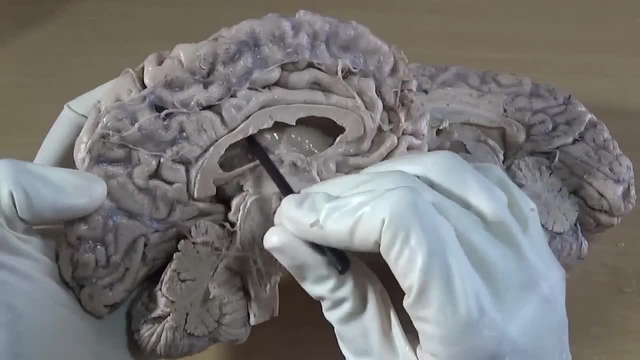 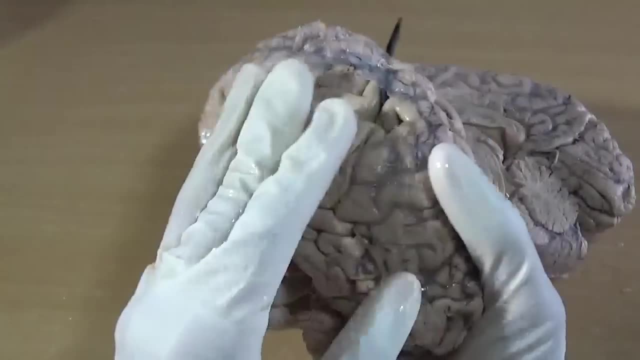 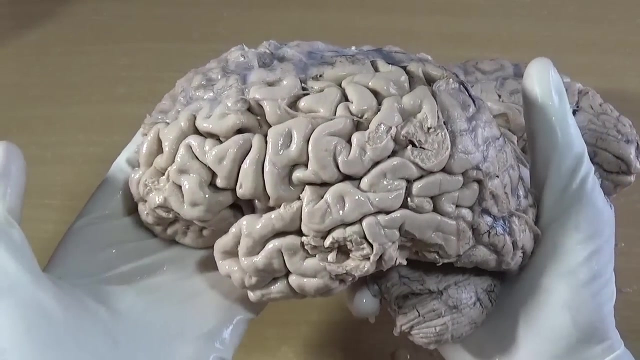 through this corpus callosum and deep inside. you can see this is the cavity, this is the lateral ventricle, that is the cavity of telencephalon. So what we are seeing right now is nothing but telencephalon and due to its tremendous growth, it assumes large surface area, say, for example, in an 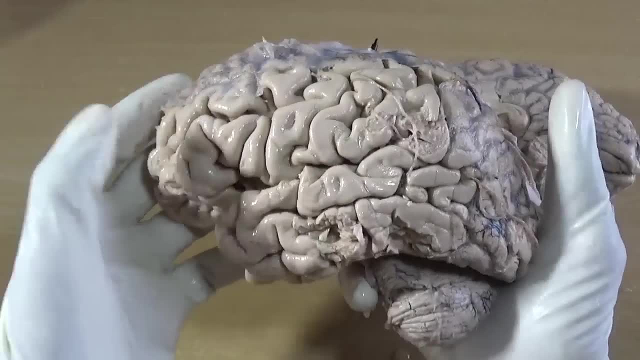 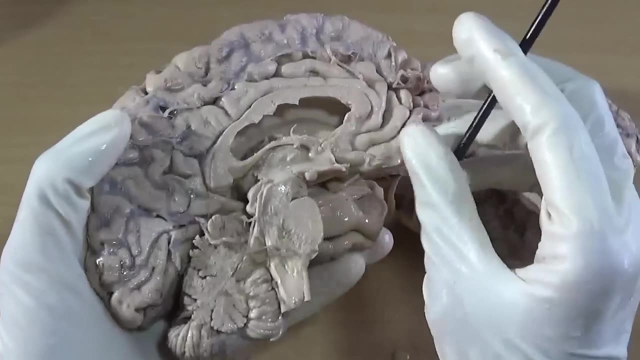 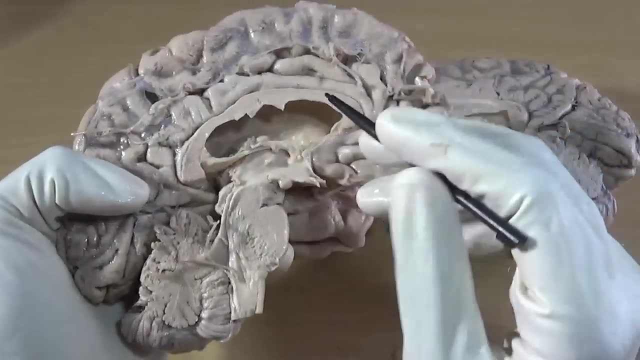 adult. on an average the surface area is 2000 square centimeters and to accommodate this much of surface area, obviously it has to convert into sulci and gyri and that's why it turns out to be gyrencephalic. So this is the cavity of telencephalon, that is, lateral ventricle. Previously we also discussed cavity of. 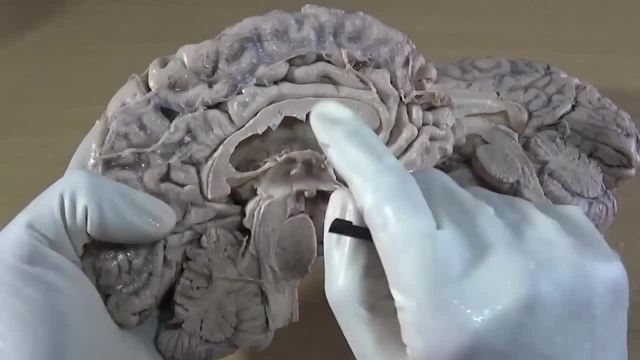 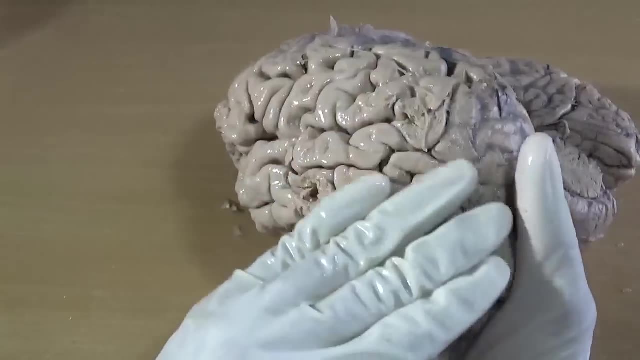 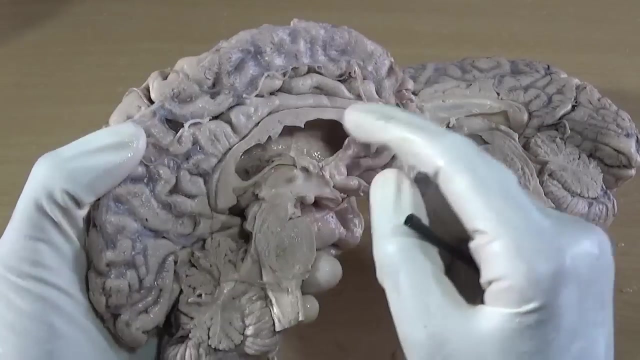 the diencephalon. that is third ventricle. So this is nothing but telencephalon and it is having, as we have discussed, it is having outermost cerebral cortex. that is gray matter. then deep inside will be the white core and still deep inside there will be basal nuclei. that is gray matter. So when we take a 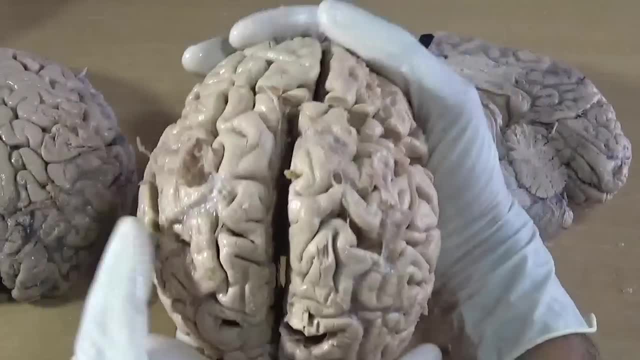 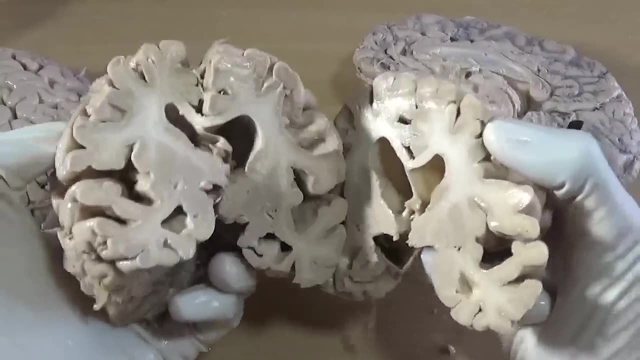 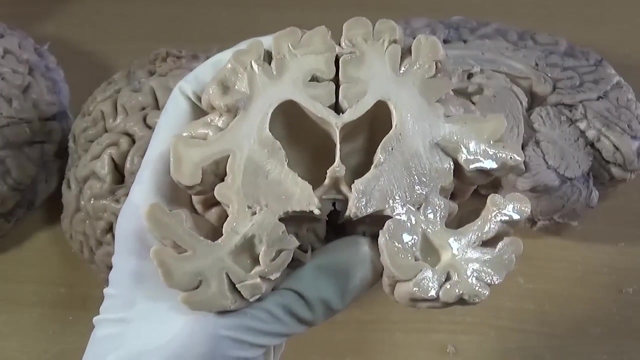 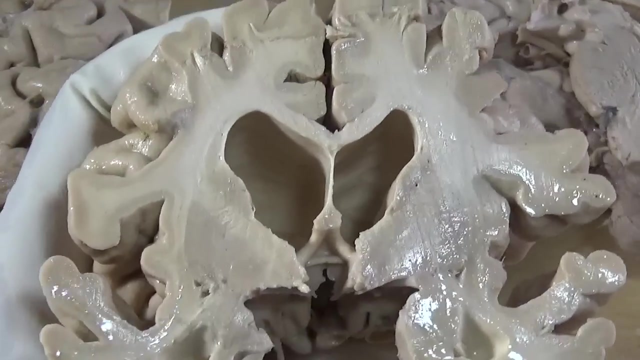 coronal section. see this instead of sagittal section. when we take a coronal section and when we see it from within, just this is how it looks like. Let me zoom in a bit. So this is how it looks like. so outermost is the gray matter. this is in the form of cerebral cortex. 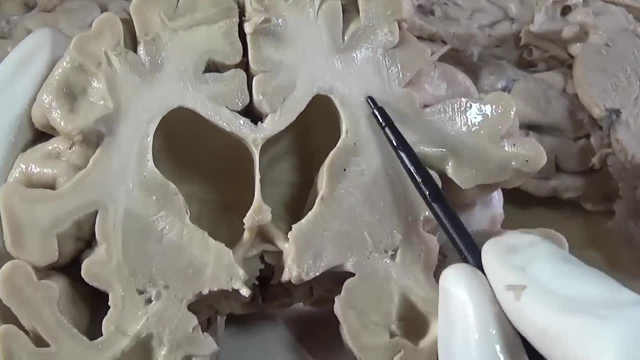 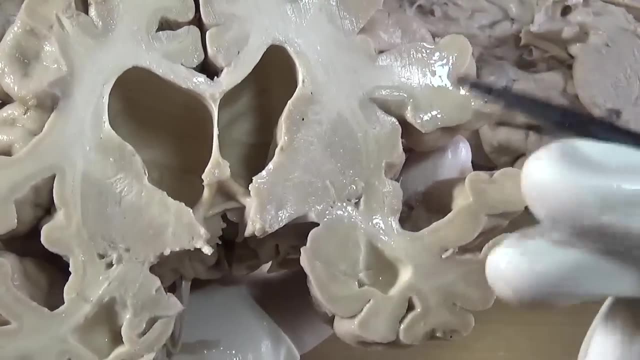 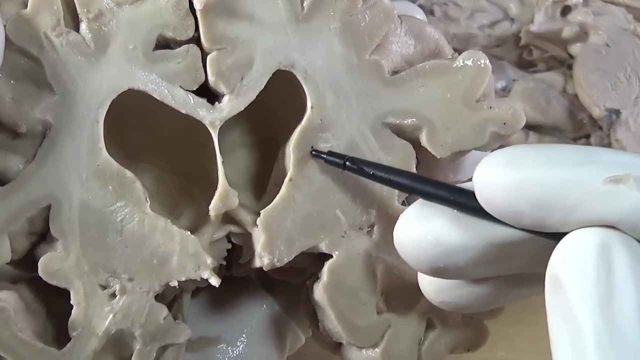 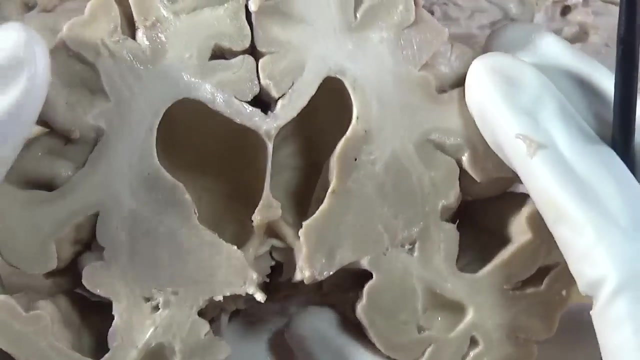 Then this is the white matter, even really make out. this is the cavity of lateral ventricle, cavity of the telencephalon, and here you can easily make out the gray matter. that is Basile nuclei, that is immediately marked as T. That is Basile nuclei that is in the form of caudate nucleus, lenthiform nucleus and certain authorities. 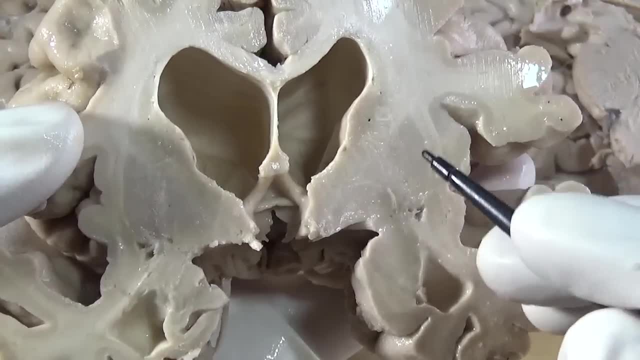 are also believing that subthalamus, so functionally, is a part of it and they believe that subthalamus- And so some of the reports that we got from others, So in fact from, of course, as often, we haveということで some medical Vienna doctors who have neuro history as well- There's a lot we know about the area in some of theseиру- Japan, for example, that you have Ramsay, for example, which have especiallyț. 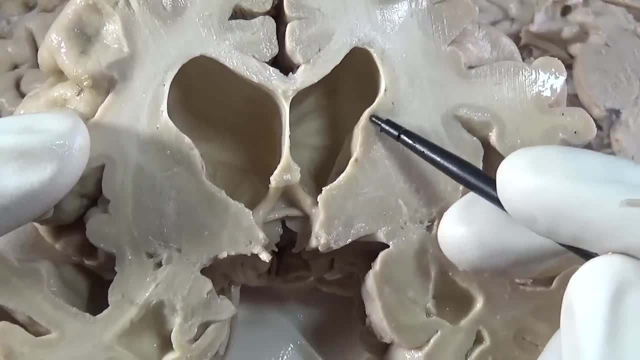 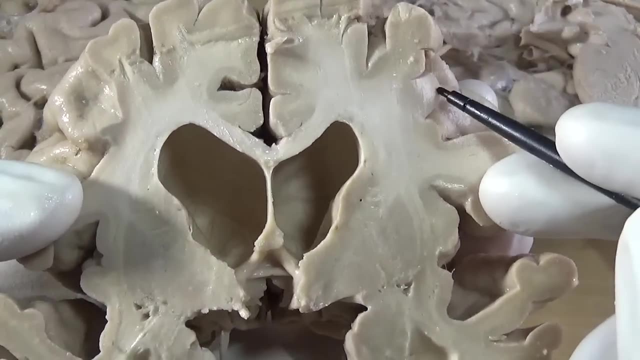 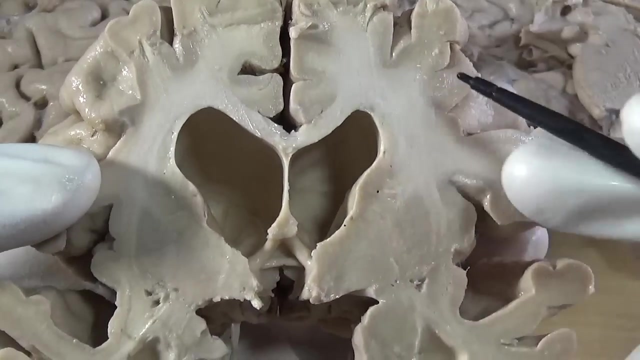 basal nuclei, but by and large you can include caudate nucleus and lentiform nucleus as basal nuclei structurally. so there is a gray matter in the form of cerebral cortex, then there is a white matter in the form of three types of fibers: commissural fibers, association fibers and projection fibers. and then 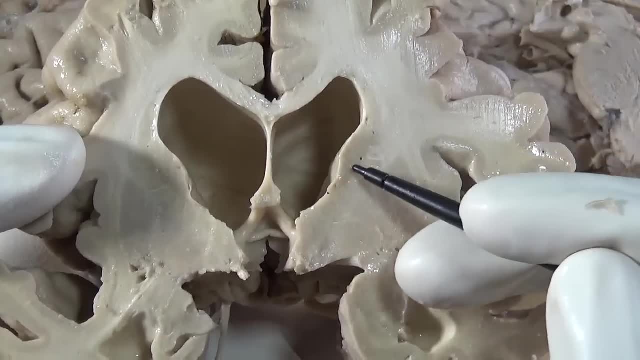 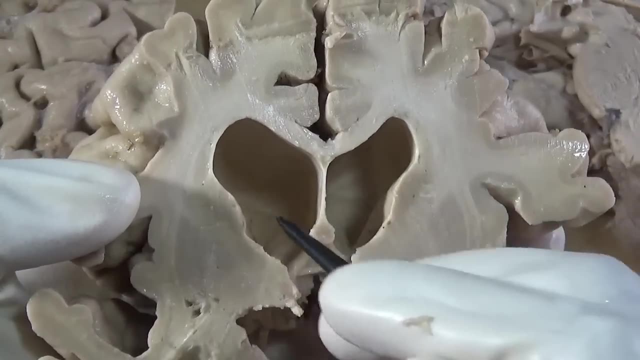 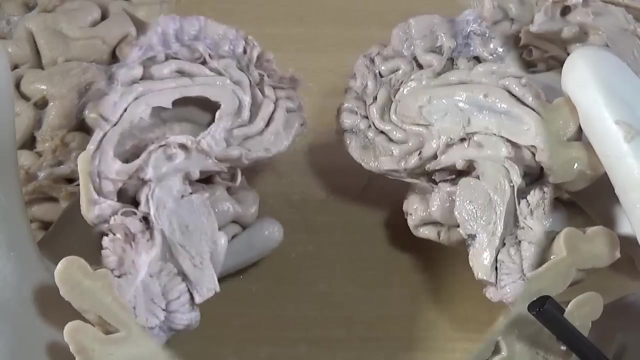 deep inside, embedded within the white core, there is gray matter in the form of basal nuclei and deep inside there is a cavity of the telencephalon. that is little ventricle. so this is how, structurally, the cerebrum or cerebral hemispheres are made. so when we discuss the external features in individual 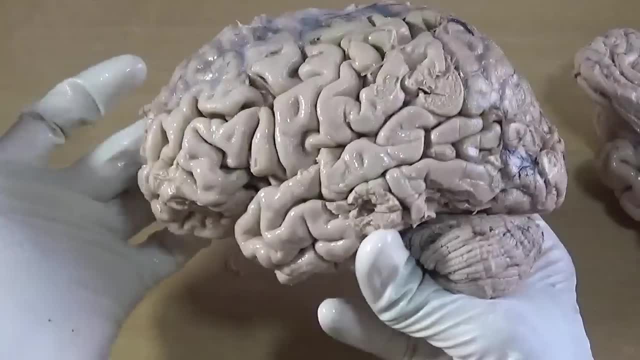 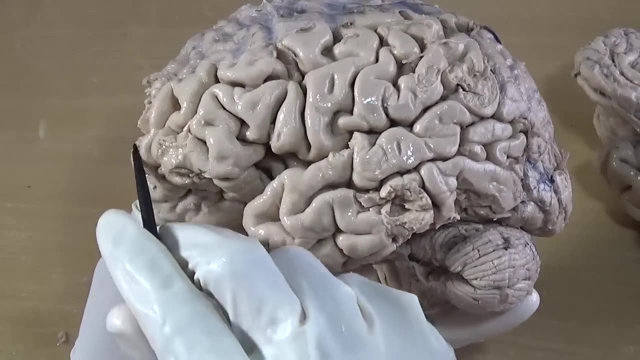 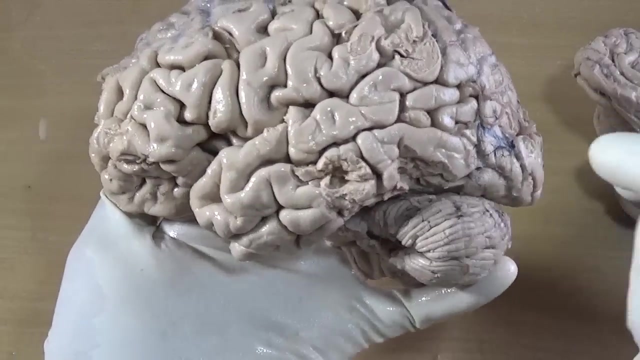 cerebral hemisphere. this is how it looks like and, as we have discussed, there are three poles: frontal, temporal and occipital. now you can clearly make out that frontal pole is more or less rounded and and occipital pole is more or less pointed. say this, and in between these two we will get temporal pole, so it is having three poles. 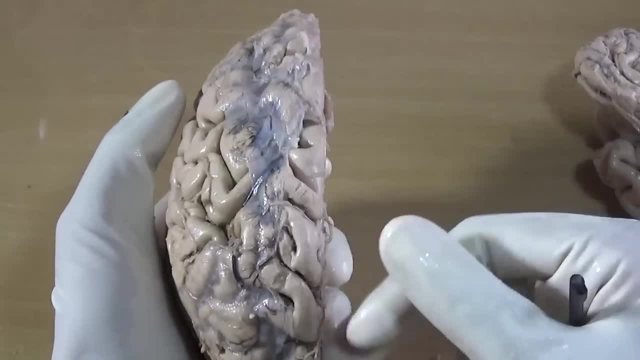 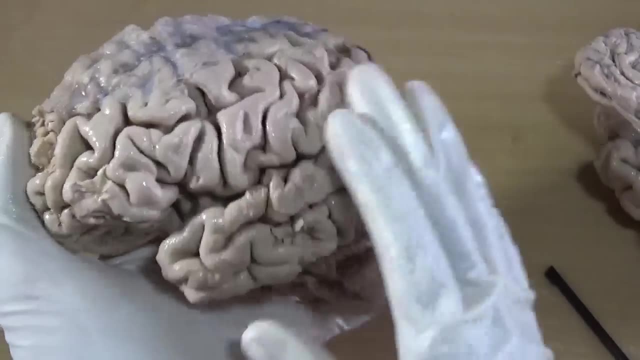 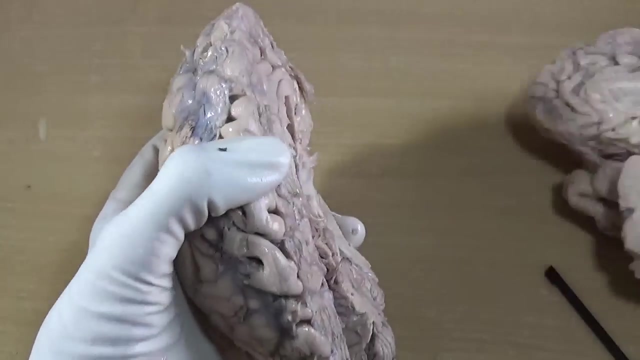 frontal, temporal and occipital. plus there are borders and surfaces. so there are three surfaces. this one is the supralateral surface and that is what we see when we open the skull cap. so this is how it looks like supralateral surface. say this when we join these two together. 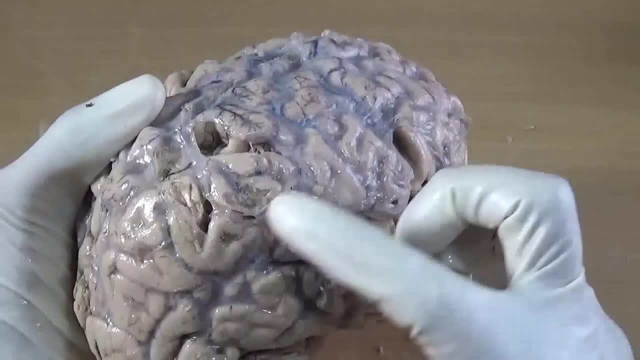 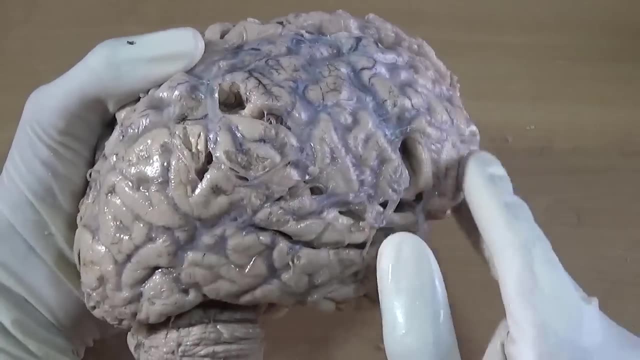 then this is how it looks like multiple sulci and gyri, and according to the sulci and gyri we can divide this surface into frontal, parietal, temporal and occipital lobes, and that we will discuss in a separate video of sulci and gyri. 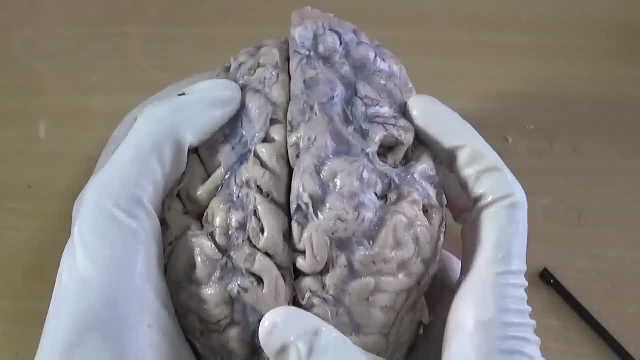 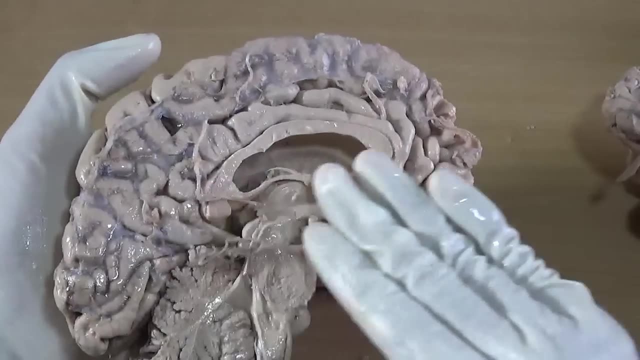 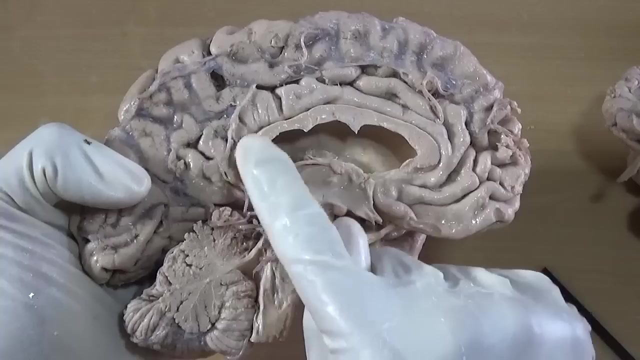 but right now you can imagine this is the supralateral surface, largest surface out of three. when we cut open, what we see deep inside is the medial surface. so this is medial surface and you can identify medial surface with the presence of cavity of lateral ventricle and particularly the corpus callosum. 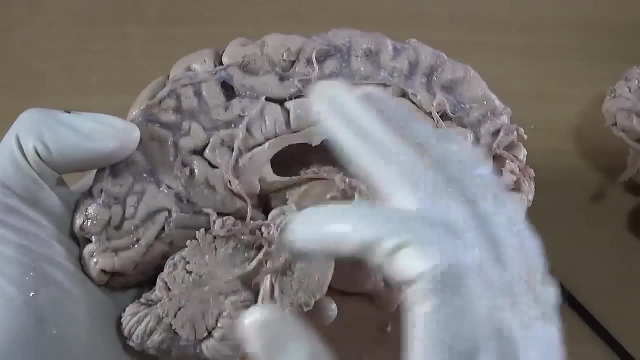 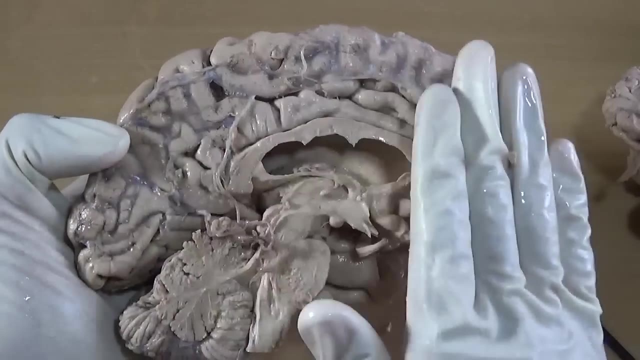 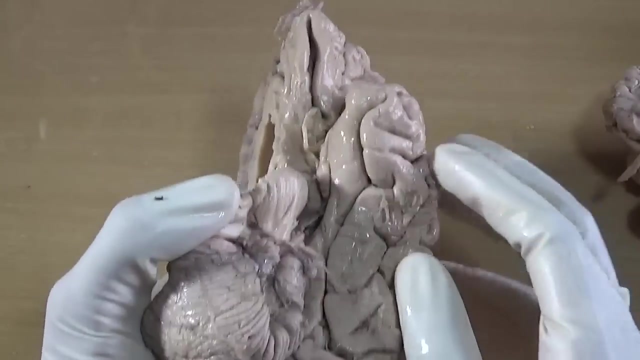 again, there are sulci and gyri and there are particular lobes like supralateral surfaces. but you can identify it with the presence of corpus callosum. so this is medial surface, this one is supralateral surface and below is the inferior surface. say this: 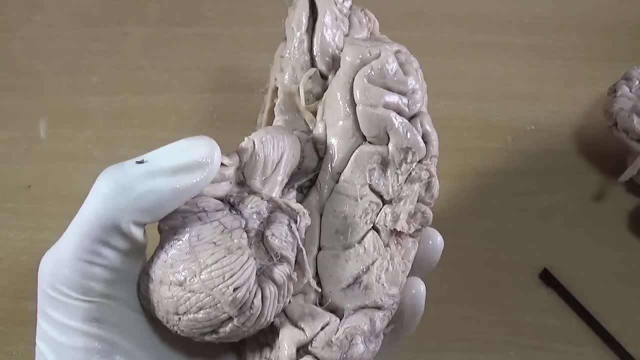 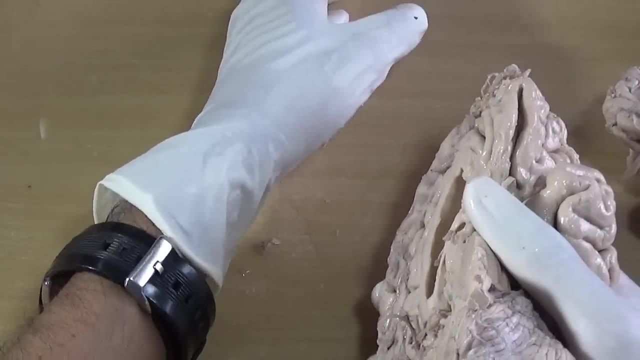 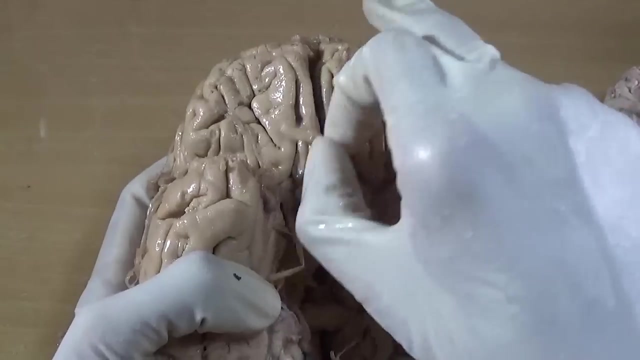 this is the inferior surface. let me show you a separate cerebrum without this brain stem and cerebellum, and then you can clearly appreciate the inferior surface. so here, this is the inferior surface. again, there are sulci and gyri and there is a presence of 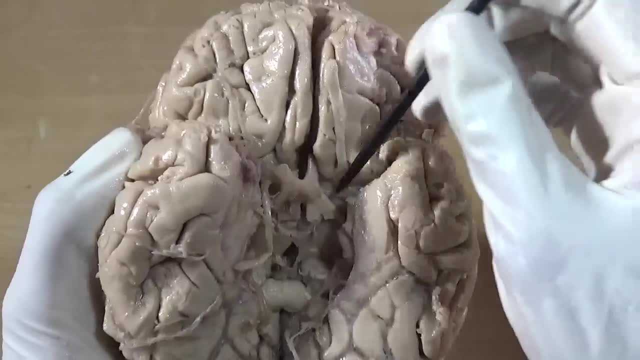 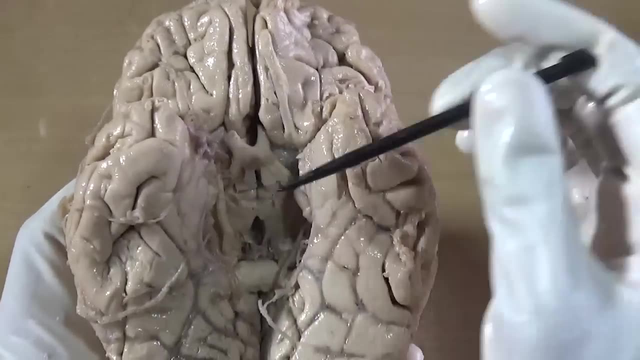 a sulcus. this is termed as stem of lateral sulcus. again, we will discuss it in a separate video, but anyway, in this case this is the space we are talking about. so this is tremベ and it is basically like stem of lateral sulcus. let me show you the bow area. 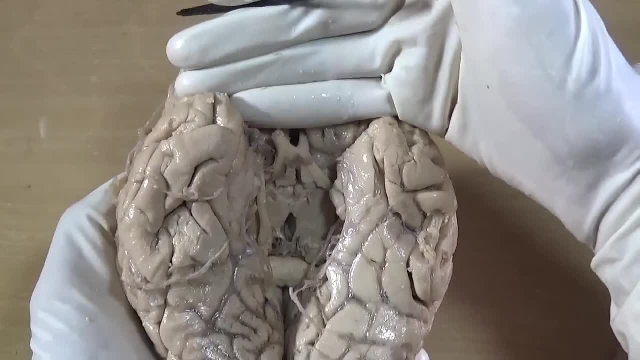 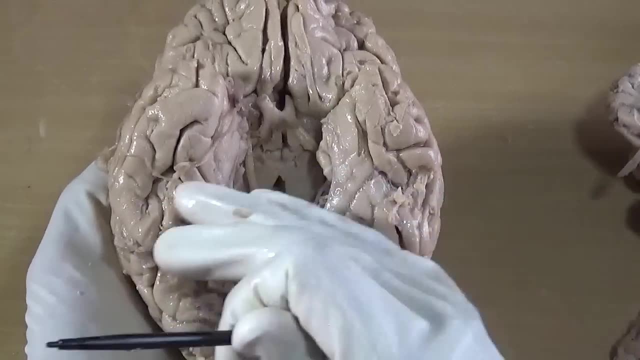 now let me show you theacre blow area. then, afraid of мин soleum, this is the, this is stem of lateral sulcus and with the ch одну, and this divides the entire inferior surface into orbital surface. and teensOh, delicious, okay. so if you have sources divided into two subcategories, 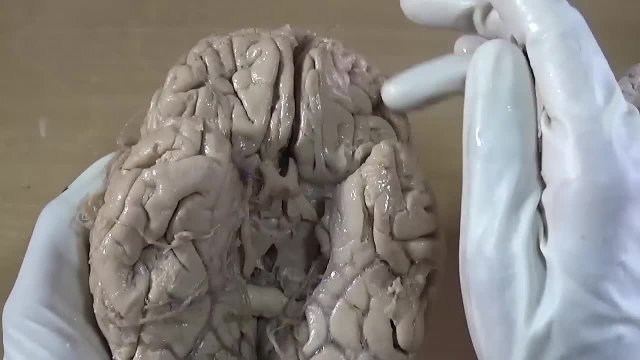 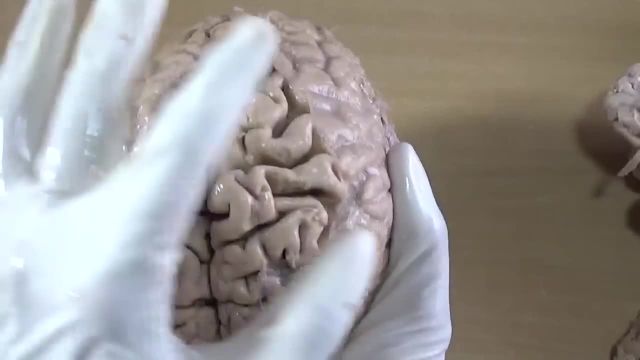 of ceremony, service and suddenly service. why this force to your, how far off distance and surface rate on that and thenству rineffectively will rest within the anterior cranial fossa, so this is inferior surface, this is supralateral surface and deep inside we will get medial surface. so it is having three poles and three surfaces. 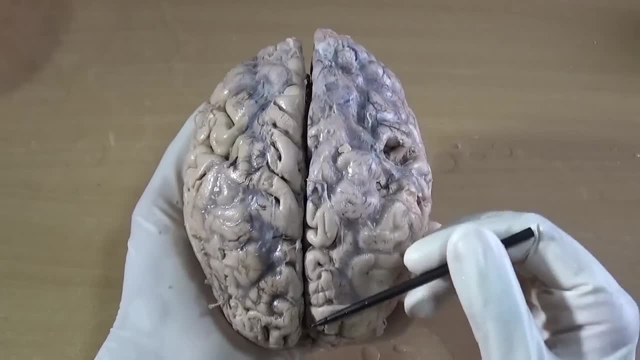 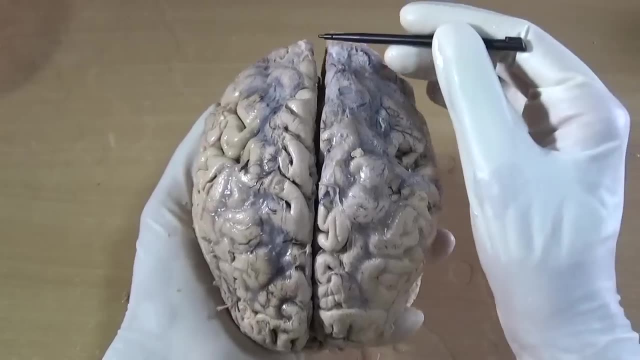 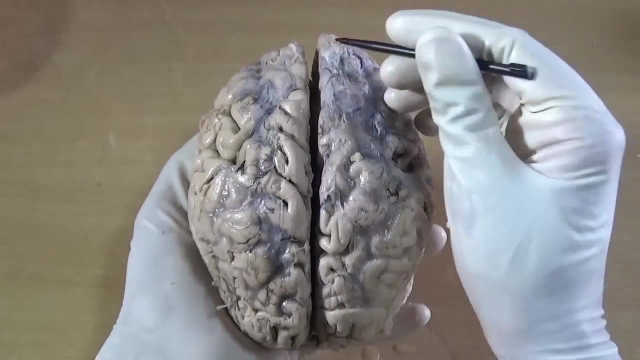 now let's see borders. now there are six borders and to remember these six borders you need to remember a pattern like one, two and three. so number one is supramedial border. this is along the supramedial aspect of each cerebral hemisphere. so for each cerebral hemisphere, this one is the 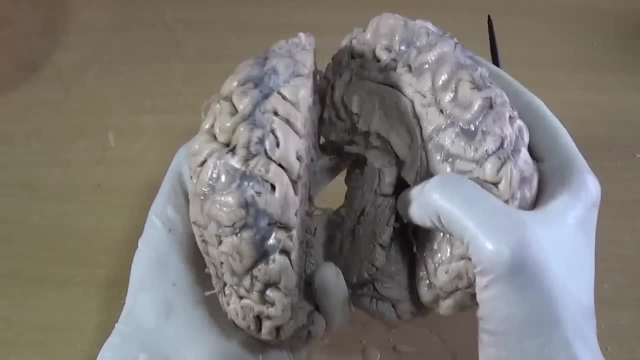 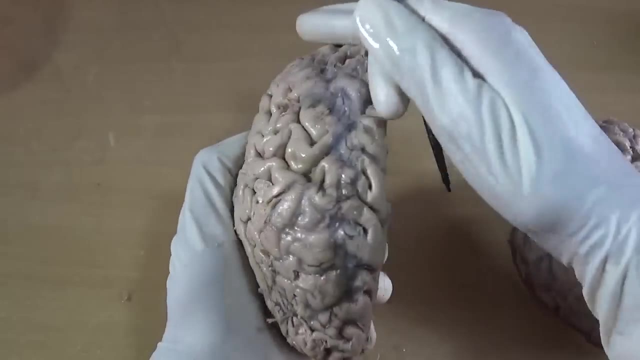 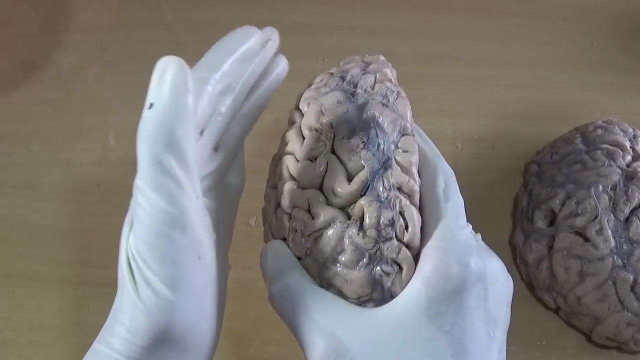 supramedial border. okay, and let me just separate these two. so here is the supramedial border and that separates medial surface from supralateral surface. very easy to remember. this is supramedial border. next is next pattern you need to remember is two. so one, two and three. two is what two is. 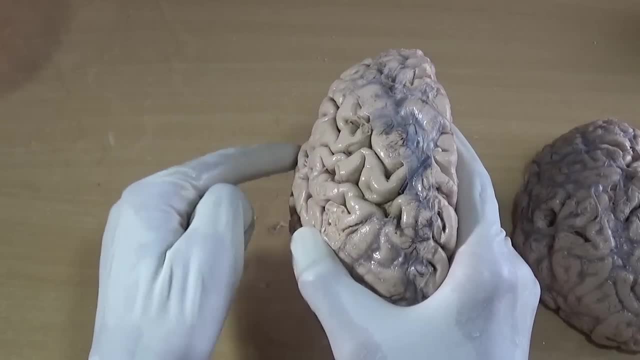 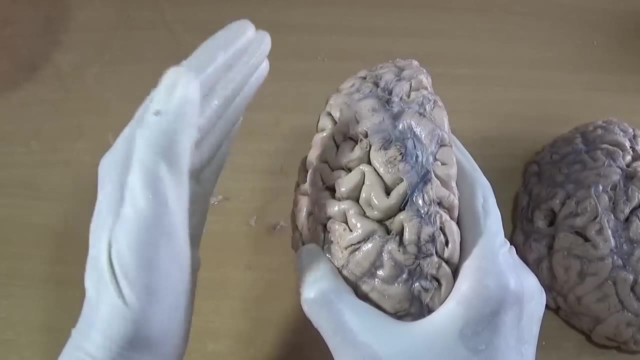 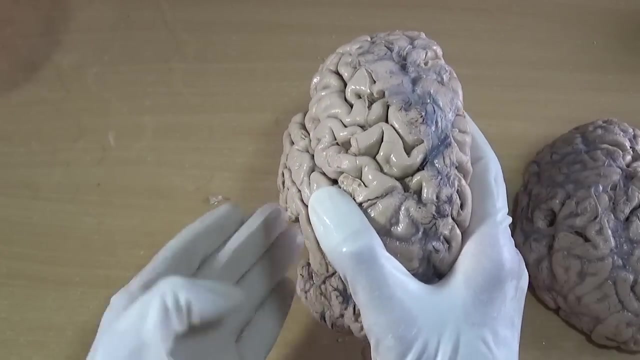 along the infralateral aspect. so, along the along the infralateral aspect, you will get two borders. this one is the super ciliary border and that separates inferior surface or orbital surface from supralateral surface, and this is the infralateral border that separates tentorial surface from supralateral surface. so, along the 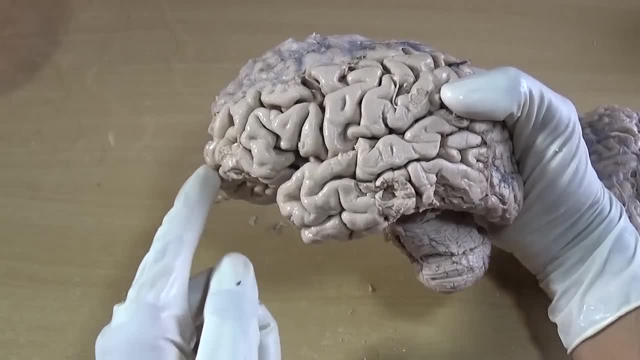 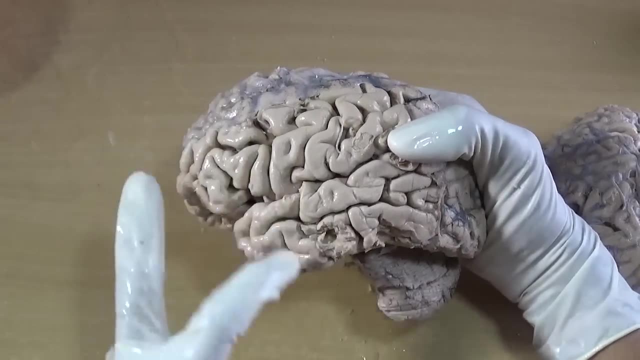 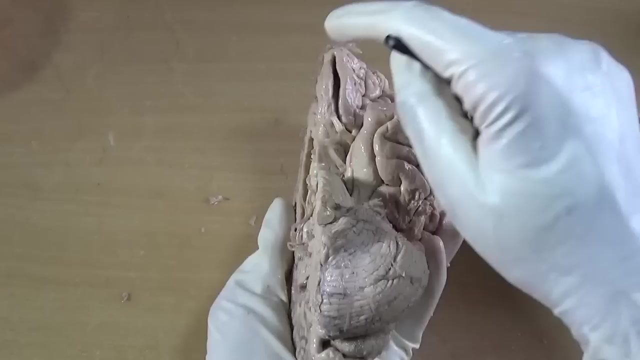 lateral side. this is the super ciliary border and this one is the infralateral border. so one is supramedial border, two are super ciliary border and infralateral border, and below you need to remember three, that is, along the inframedial aspect. there are three borders. this one is the 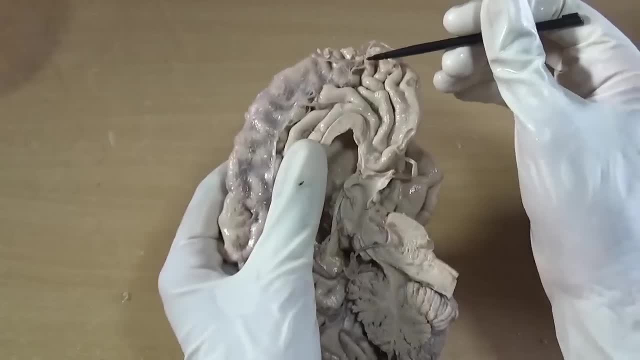 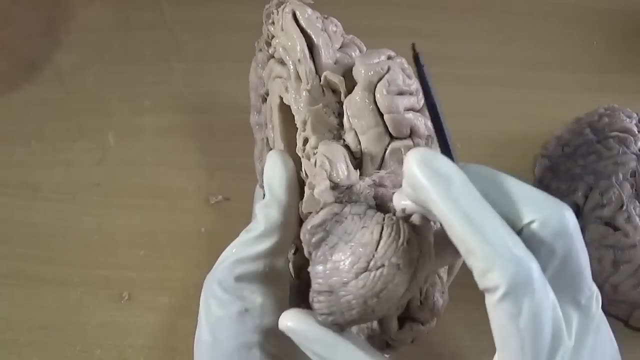 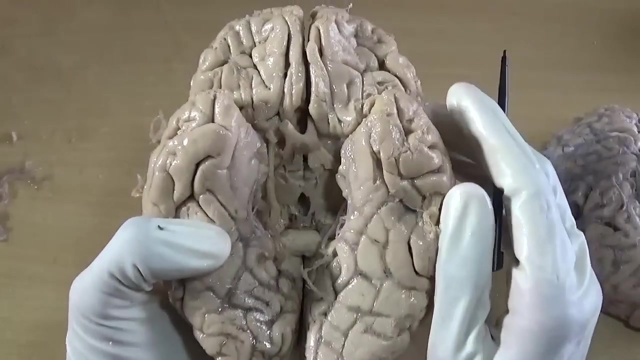 medial orbital border that separates medial surface from orbital surface. say this: second one is the hippocampal border. let me show you a separate cerebrum. say this. so here the brain stem and cerebellum has been removed, so what you can see is this is the.